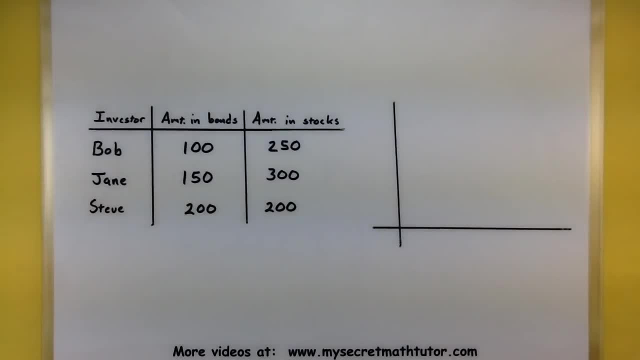 those relationships Like? does it look like people are investing more into bonds or more into stocks? Well, we could look at the data in the table, but it'd be much nicer if I could just quickly look at, say, a chart and be able to figure out that same information. 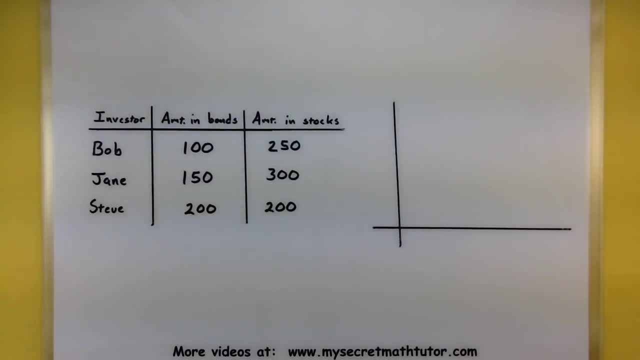 So let's take this and now put it into a nice, more visual thing using a nice little chart. over here We're going to do a bar chart, So I want to list out my three investors. I got Bob, We'll do one for Jane, And let's 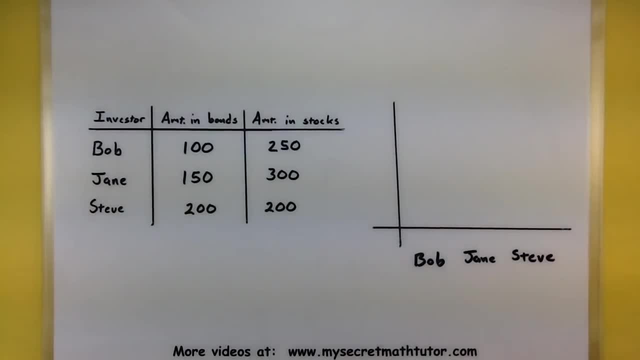 see one for Steve, Okay. And then we want to represent the amounts of money they have in each of these. Looking at the amounts, it looks like maybe going from 100 all the way up to 400, that should be good enough. So 100, 200, 300, and 400. 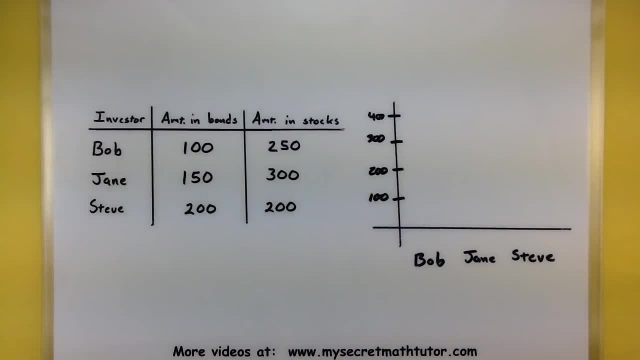 Now we want to show the two types of things that they're investing in: their amount in bonds and the amount in, say, stocks. Let's go ahead and make a key somewhere to see what we got. So we're going to do blue: We use this for bonds. 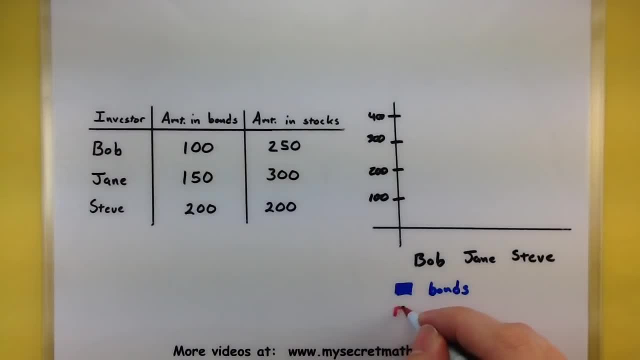 Let's go ahead and use our red one. We'll say that's stocks. Now we can create a bar for how much they have in bonds, how much they have for stocks, and we'll be able to visually see what they have. Let's start off with Bob. 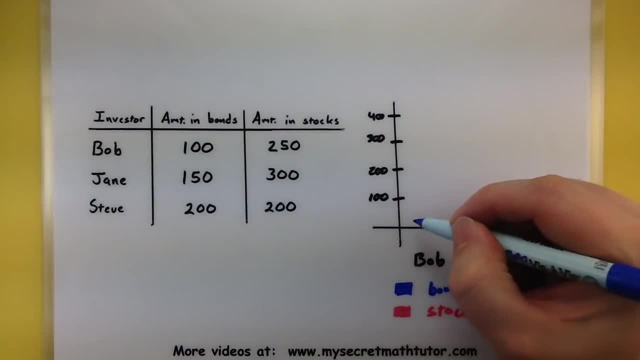 So, starting with Bob, looks like he has $100 in bonds, So we'll make a small bar goes up to the 100 mark and back down. So now you can visually see how much Bob has. Let's see for Jane. we have even more in bonds So we'll do a larger one that goes. 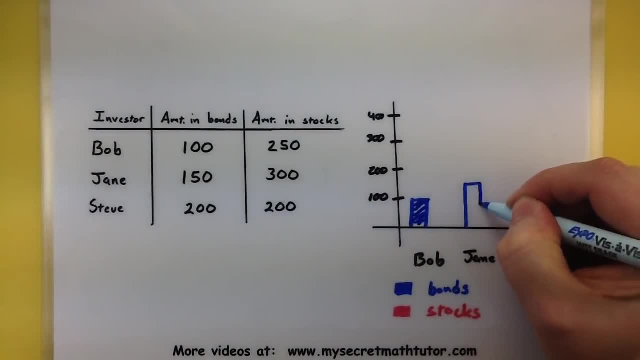 halfway between 100 and 200.. And quickly, I can see that Jane is definitely going to have something in bonds. Let's go ahead and click on the line and go to the top of this bar And we'll see that this is the number I need to go in. In a minute I'll be able to see that I have 100. And if you're.